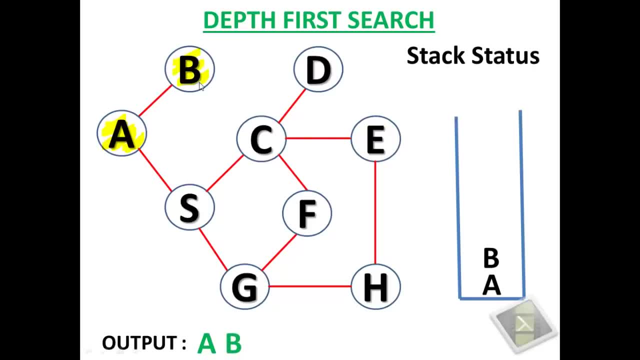 Now, B being at the top of the stack and A as only adjacent visited node, there is no other go, So we will pop up from the stack B. Now we have A at the top of the stack and S as the adjacent unvisited node, So we will push S to the top of the stack and we will 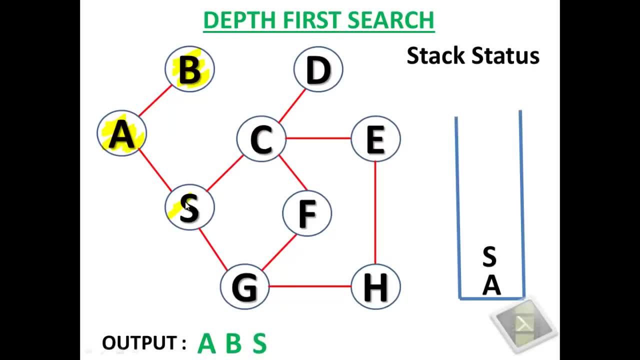 add it to the sequence Mark. it as visited Now S at the top of the stack and C and G are the two adjacent unvisited vertices. Alphabetically, we will push C on the top of the stack and add it to the sequence Mark. 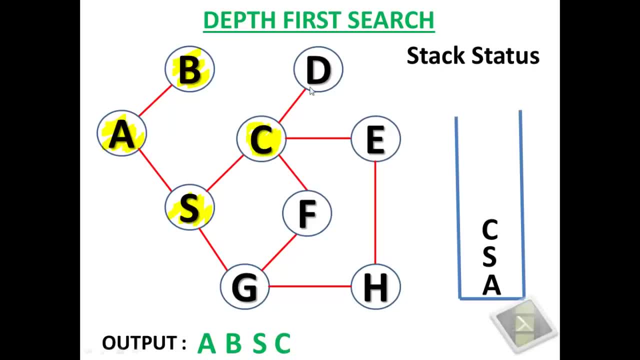 it as visited. C has D, E and F as adjacent unvisited nodes. So alphabetically we will push D on to the top of the stack and add it to the sequence and mark it as visited, D being at the top of the stack with C as the only adjacent but visited node. So there, 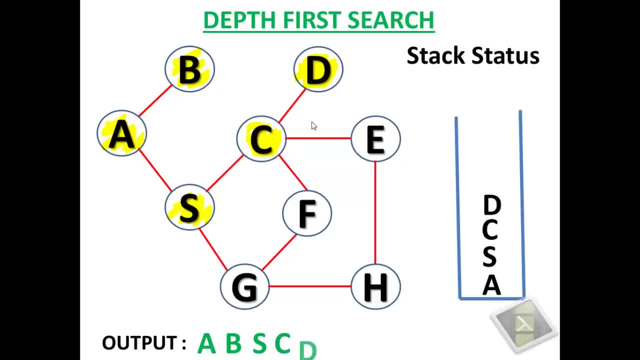 is no other go, We will pop it up from the stack. Now we have C at the top of the stack and E and F as the adjacent elements of C, So we will push E alphabetically first and add it to the sequence and mark it as visited. 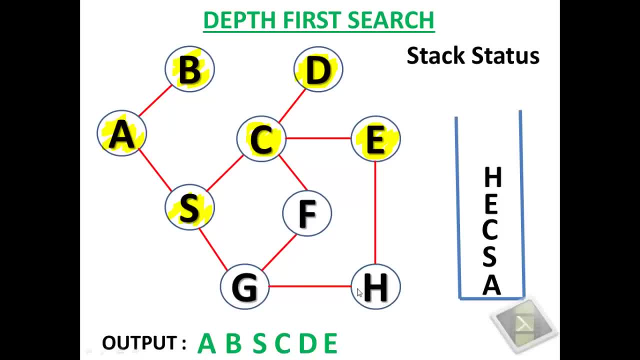 H as the adjacent element which is unvoited. We will push it to the top of the stack and we will add it to the sequence, Mark as visited. H has G. so we will push it to the stack and add it to the sequence and mark it as visited. 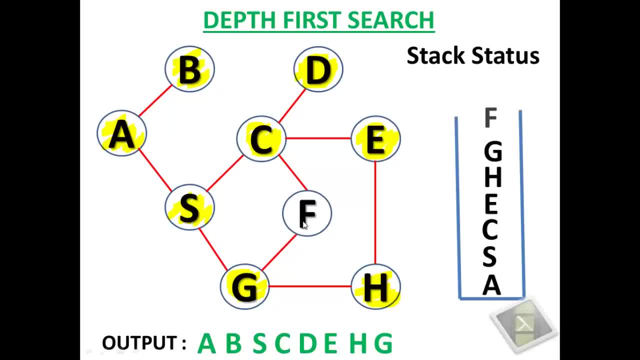 And at last we have F, we will push it to the top of the stack and add it to the sequence marking it as visited. Now F, as is the top symbol of the stack, and f has both c and g as visited nodes and adjacent nodes, so we will pop it off. 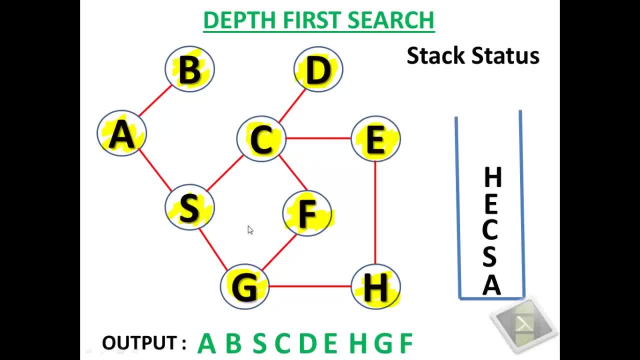 Similar is the case with g: we will pop it off. Similar is the case with h, e and c. So we will pop h, e and consecutively c. Same is the case with a and we have reached last symbol of the stack, and that is a, So we will pop it off and that's it. Stack is empty.